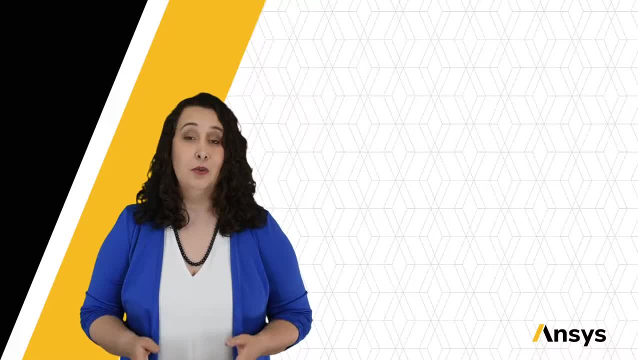 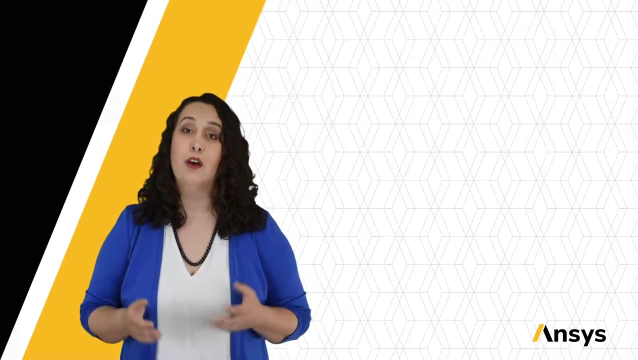 So let's get started. Aluminum is also one of the most common elements found in the Earth's crust. yet we never find aluminum ore on its own. Instead, aluminum is always mixed with other elements. Bauxite is one of the aluminum ores that we commonly use to get pure aluminum out of. 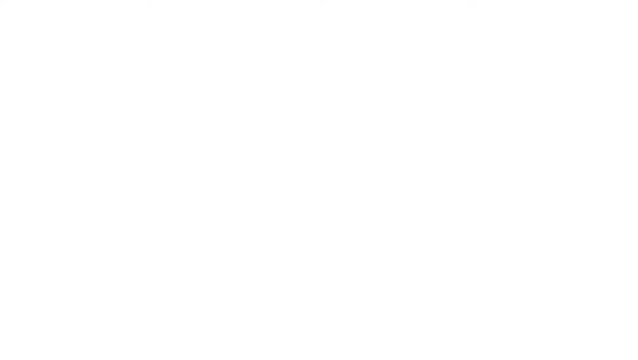 It exists in a mostly hydrated aluminum oxide state. To get from our bauxite to aluminum, we use what's called the Bayerring. It's a very simple process. First we grind and calcine our bauxite. Then it's treated with sodium hydroxide at high temperatures to convert our aluminum. 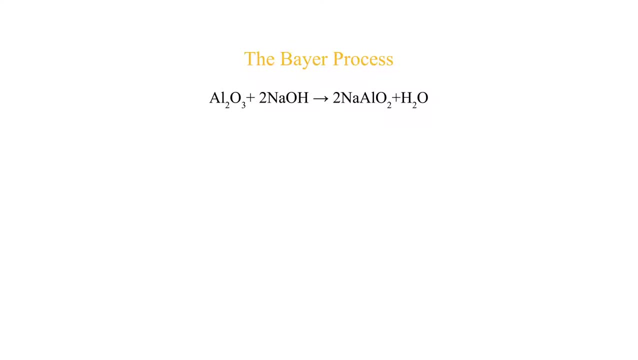 hydroxide to sodium aluminate. After removing impurities and other undesirable byproducts of this reaction, we slowly cool our solution to precipitate out aluminum hydroxide. We then wash this, heat it up to 1100 degrees Celsius and finally get aluminum oxide. 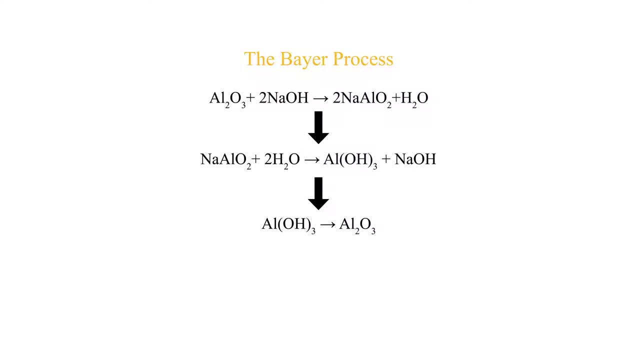 This process is called the Bauxite. We can now take this much more pure aluminum oxide and dissolve it in a bath of molten kryolite. Now we use an electrochemical process to deposit almost pure aluminum. The purity we get is von 99.5 to 99.9 percent. 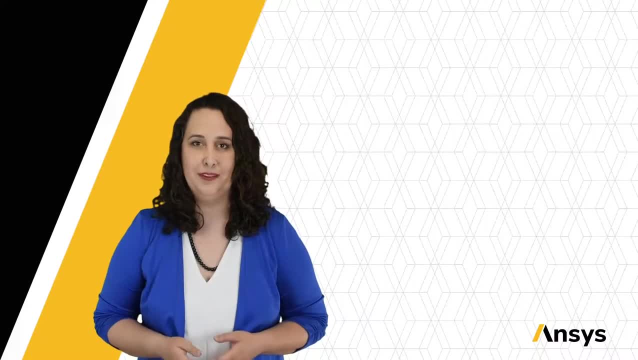 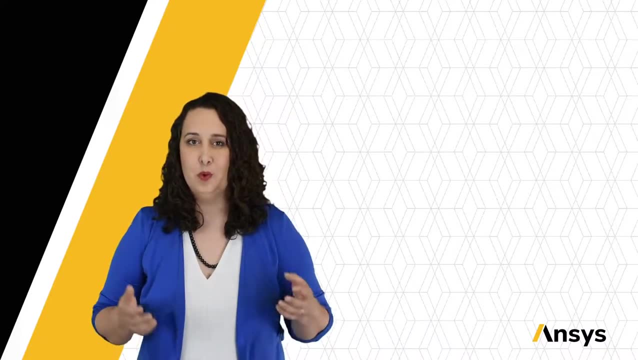 This is very time consuming to go from bauxite ore to pure aluminum. And that's not the end of the story. Just give the bauxite ore some more time, I'll get you back. It's actually less energy intensive to recycle aluminum and get our pure aluminum back. 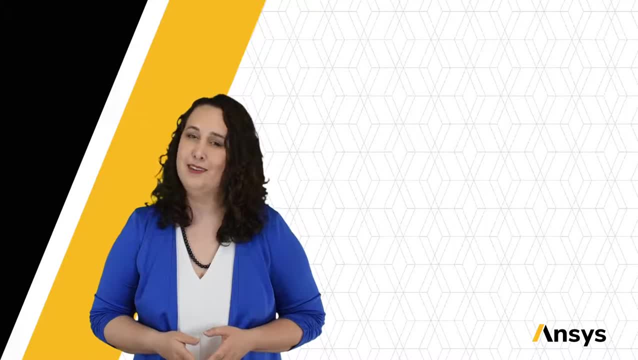 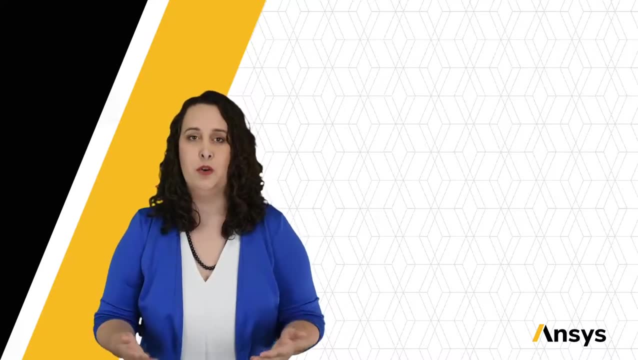 We'll learn more about these things in lesson three, but it's all the more reason to keep recycling. So now we've completed stage one. We have a usable starting material, whether it's our pure aluminum, our polymer monomer we got from crude oil or a carbon fiber. 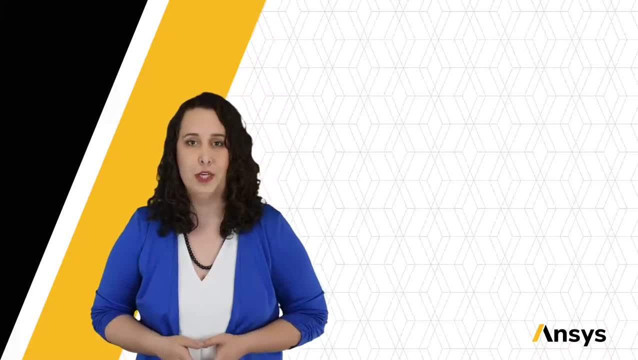 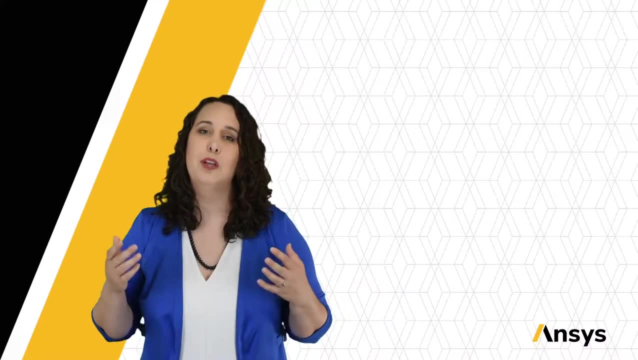 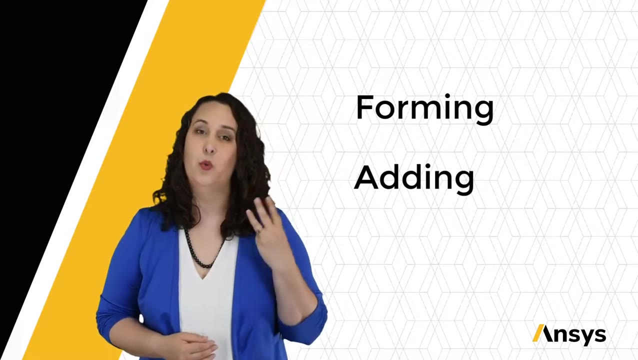 Now we can move on to stage two, our processing operations. Once again, there are going to be multiple steps in our processing operations, but in this stage we're generally using one of three approaches: We're forming our material, we're adding material or we're subtracting material. 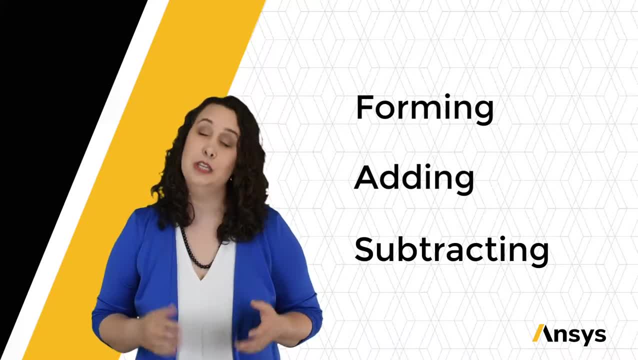 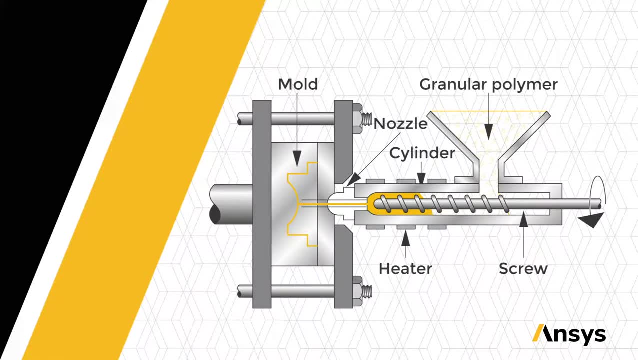 Regardless of which approach you're picking, you're somehow altering the shape of your material. Let's start with forming. If we're forming our material, we're somehow defining the shape our material should be. An example of this is injection molding, Used to make a variety of polymer parts. 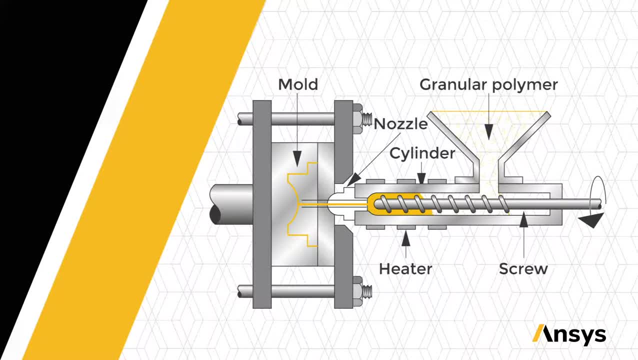 In this schematic we see that our starting material is some type of polymer powder. This is pushed through our screw nozzle and melted, And this melt is then pushed into our mold or injected. This mold will define our product shape. As the part cools within the mold, the shape is maintained. 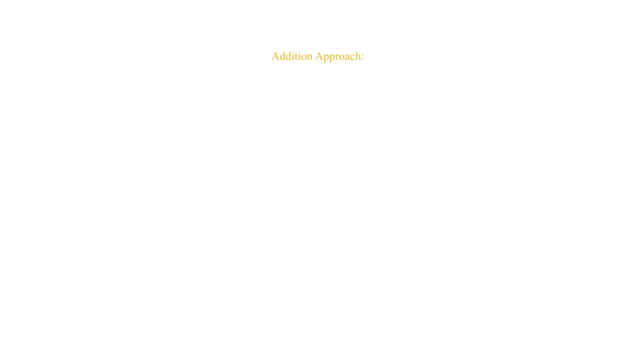 The next approach is addition. You may be familiar with this already. This is Additive manufacturing. If a print head is used, it can be called 3D printing. Additive processing involves starting with no material and adding our starting material through various techniques to finally end up with our part or product. 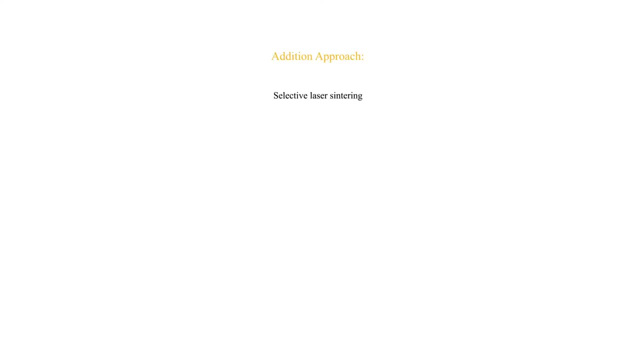 We can see an example here of selective laser sintering, which can be used with both metal and ceramic powders. We start with a substrate submerged in a bath of our starting material, In this case a metallic powder. A laser We'll sweep over the material, solidifying a layer of our powder. 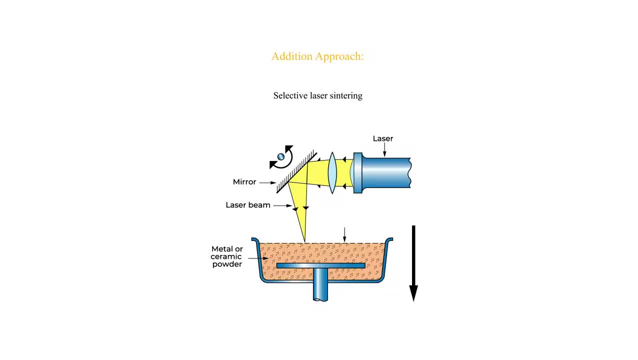 The substrate will then move down a specific distance, allowing for new, fresh powder to flow over the top of our part, And then the laser will pass over again. This allows us to build up our material layer by layer. Additive manufacturing is highly sought after for its rapid prototyping capabilities and minimal material waste. 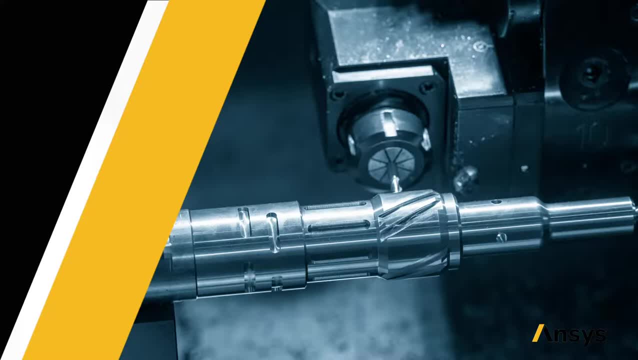 Finally, we have the subtraction approach. To me, this is a classic way of doing things. Think of carving a piece of wood, maybe for a bowl, a decorative item or a chair leg. You start with a larger piece of material than what the final part needs. 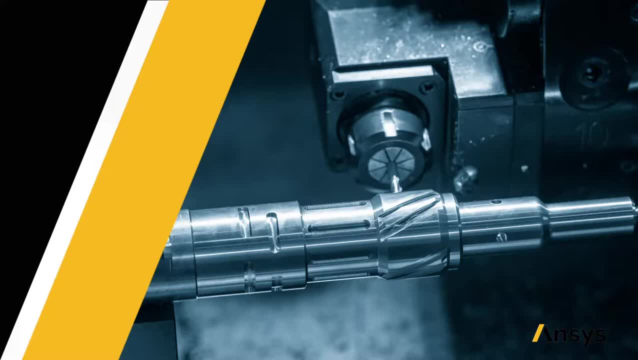 Then you subtract or remove material to get to the final piece. Maybe you're turning a piece on a lathe, cutting with a saw or chipping away with a chisel. However, the method- we subtract material to get where we need to be. 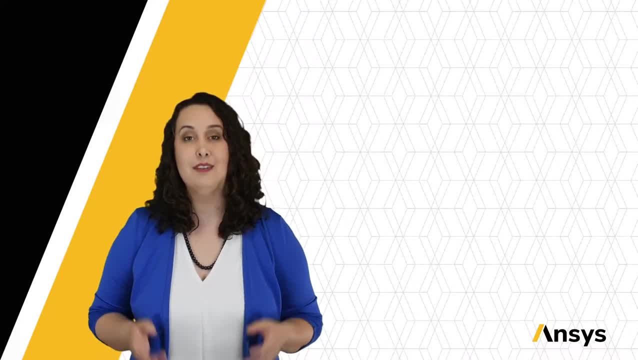 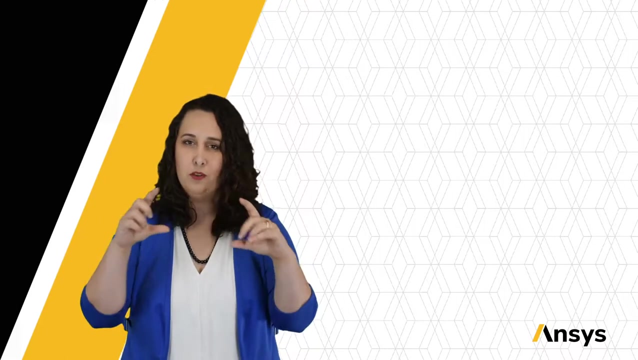 We've now completed Stages one and two. We can move on to stage three, the post-processing. Some materials might need a significant amount of post-processing, Others not so much. If I'm thinking of additive manufacturing, often we have small supports just to keep our piece stable as we're adding our different layers. 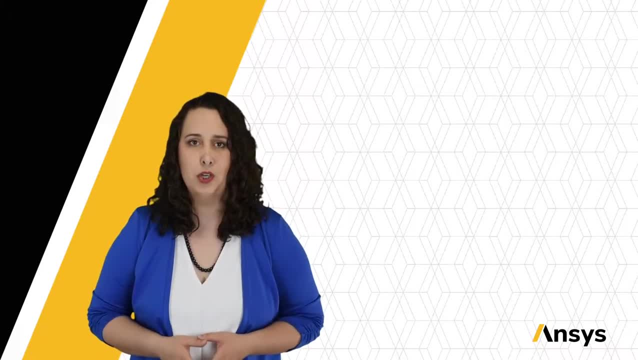 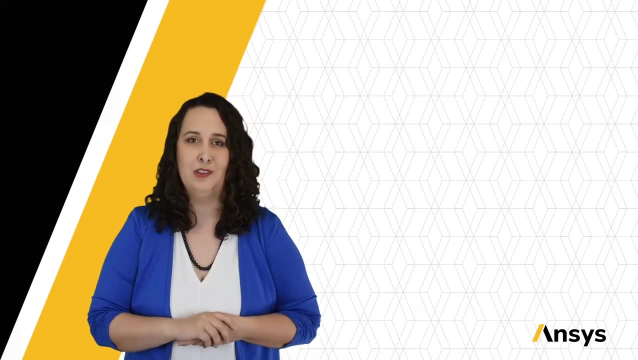 These supports can then be removed and we're pretty much good to go. In the case of our injection molding, perhaps we overfill the mold just to make sure we fit into all the nooks and crannies. We'll want to cut off the excess material from the edges of our mold. 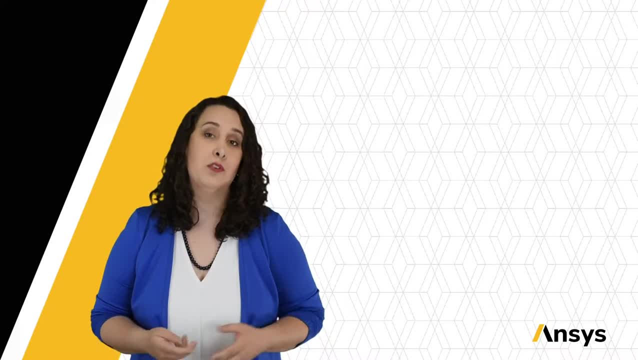 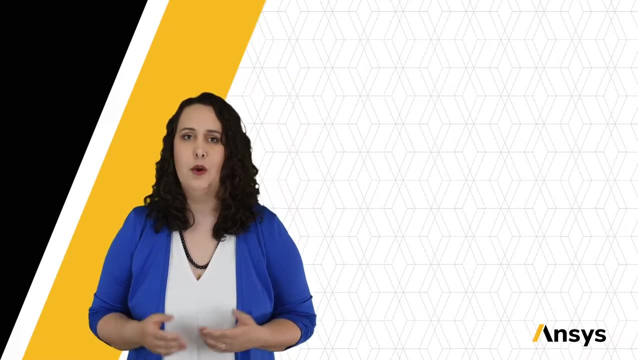 Perhaps I need to drill a hole in my part because it's going to be joined with something else. Perhaps I need some type of surface treatment or finish. I might need to polish the piece or apply a coating or paint it. Whatever the post-processing treatment, it's always chosen. 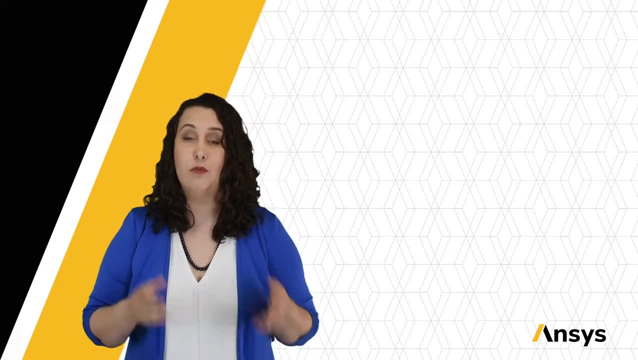 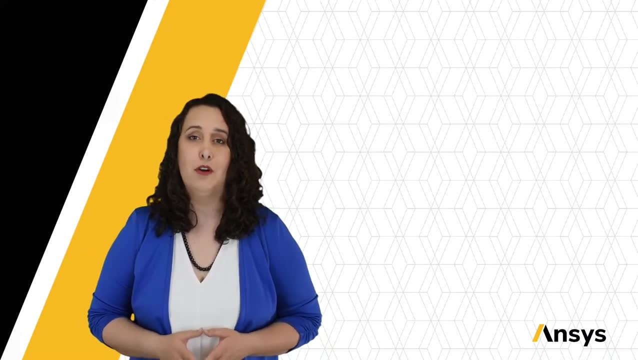 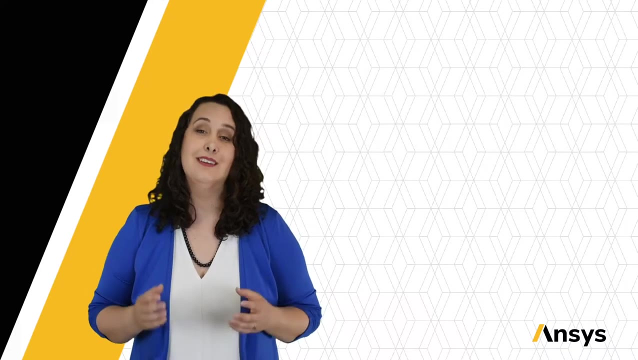 with the final way that the material needs to behave once it's serviced. And with that we've covered all of our three stages of our processing operations and gotten from raw material to a final product. Now, this is a simplified version due to the introductory nature of this course. 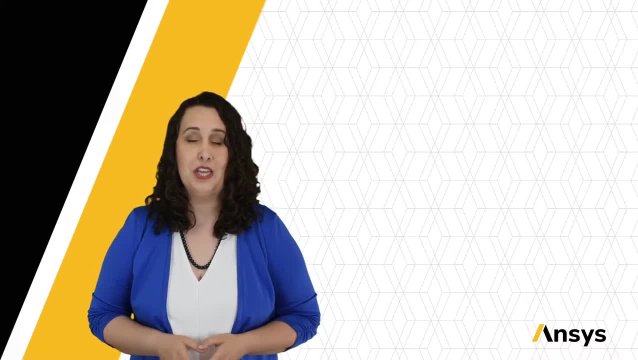 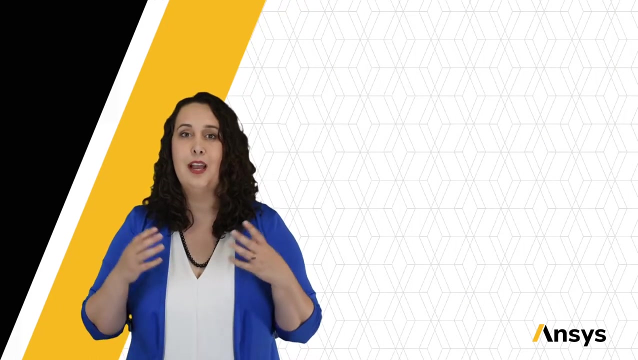 But we've seen how many different steps can go into getting from our raw material to the various products in our homes. For lesson two, we're going to be talking about four key elements of processing Time, temperature, environment and pressure, And seeing how these impact our material processes. 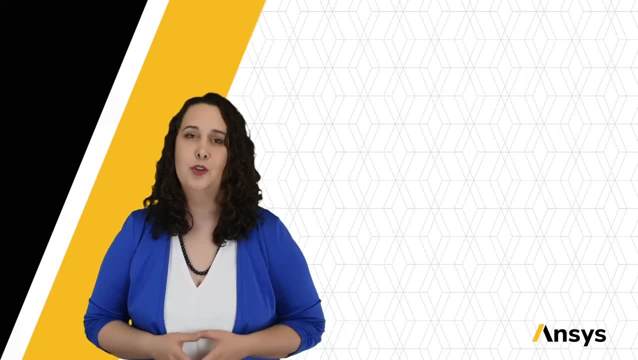 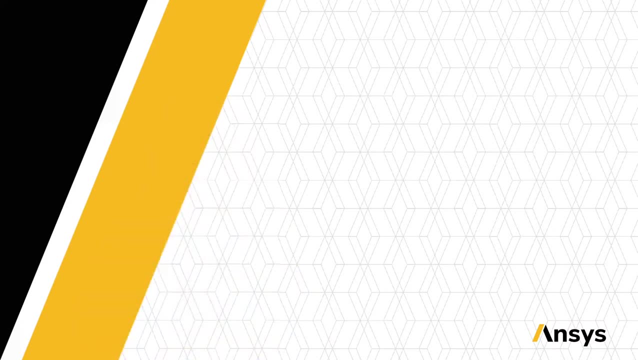 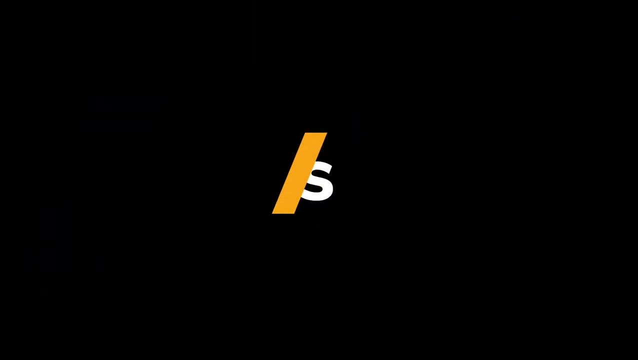 For ease of understanding, we split this into four shorter videos. So join us as we see the impact that these four little elements can have. Thank you for watching.